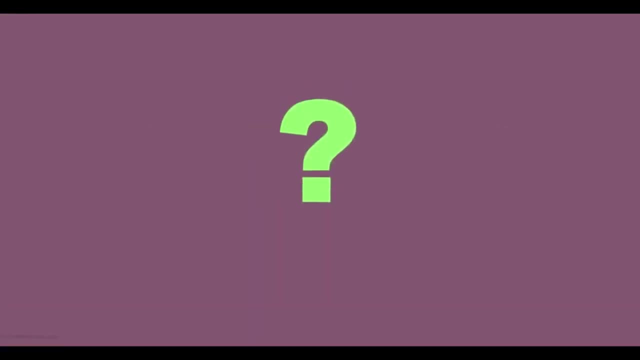 be released as a by-product. Now does this happen every time? I mean, will an acid and an alkali always give us salt and water? Yes, it will always be like this. An acid when combined with a base will always give us salt and water. And what is this reaction called? 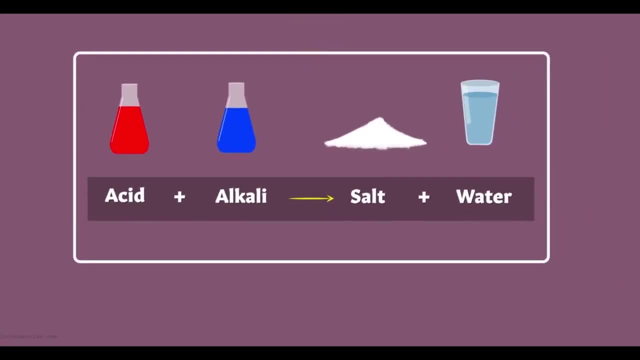 Does it have a specific name? Yes, it does. It's called a neutralization reaction. Here, the strength of both the acid and the base are lowered. They are brought to a neutral point where the intensity of the acid as well as the acid are reduced. 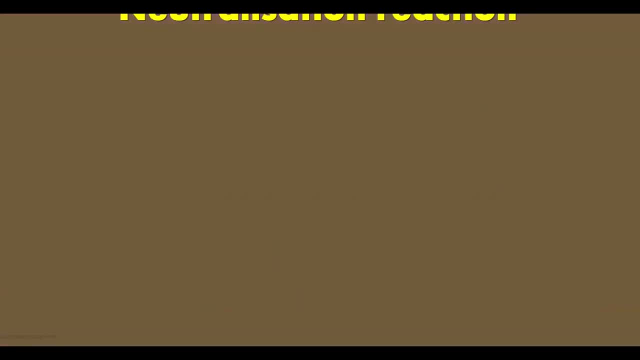 The best example to study a neutralization reaction is the formation of sodium chloride or simply put, common salt. If we take hydrochloric acid and combine it with sodium hydroxide, then the neutralization reaction gives us sodium chloride and water is obtained as a 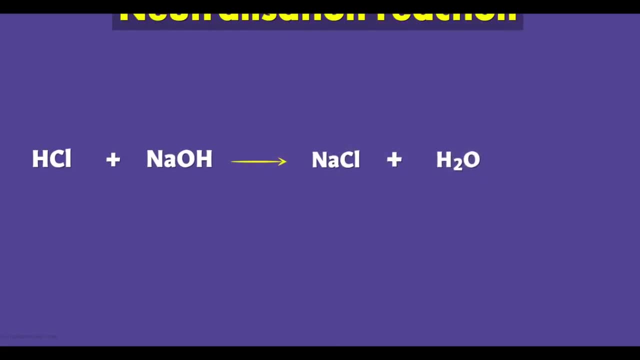 by-product. The reaction also liberates a lot of energy in the form of heat. This is how every neutralization reaction works. 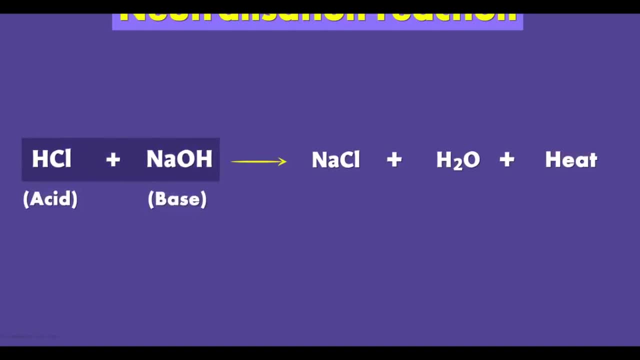 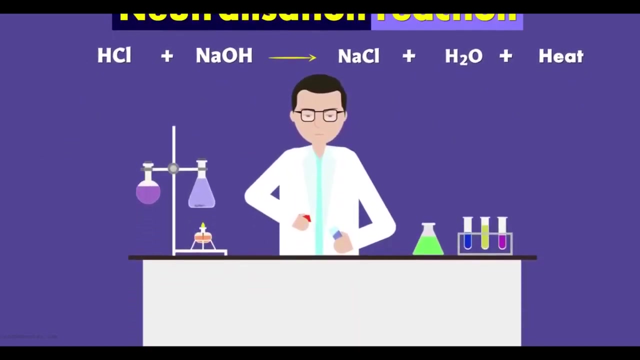 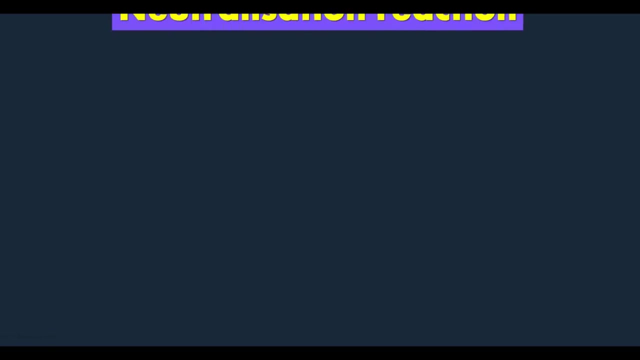 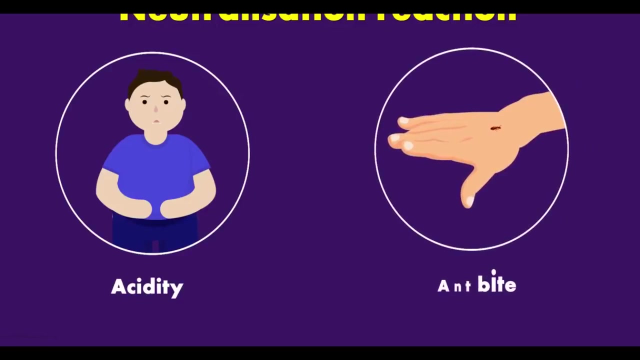 Acid and a base combine to give salt and water with heat generation. But looking at the reaction of sodium chloride formation, you may say that neutralization only occurs in laboratories. When acids and bases are combined in a test tube in a lab, it's only then a neutralization process occurs. Is that the case? Actually, that's not the case. Neutralization reactions are a part of the neutralization process. Neutralization reactions are a part of our daily lives as well. Many reactions occurring inside our body or even throughout the day are neutralization reactions. For example, we usually find elders complaining about acidity. Or ants biting us on the skin. These are examples where the percentage of acid increases inside or on the body compared to the normal value. Such cases are treated with medicines. But have you wondered how How these medications work? Needless to say, they work based on the principle of neutralization. 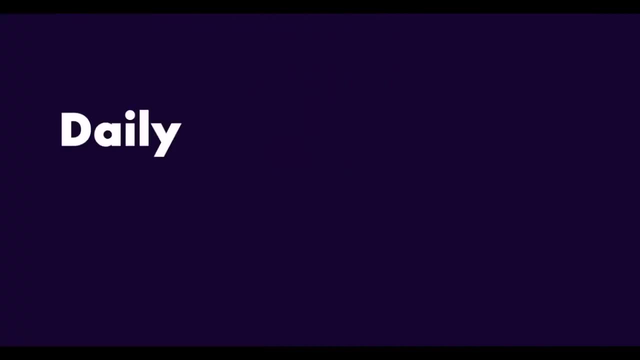 Next, let's have a glance at the various examples of neutralization reactions in everyday life. 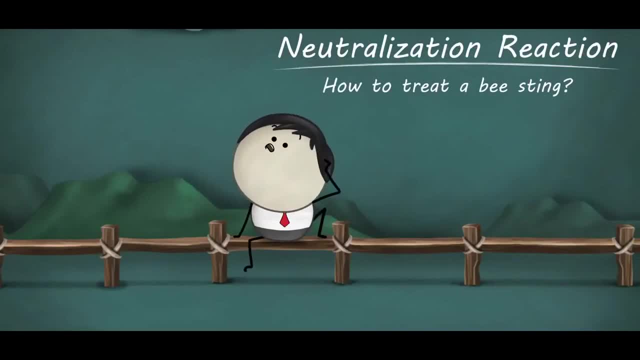 Neutralization Reaction – How to treat a bee sting 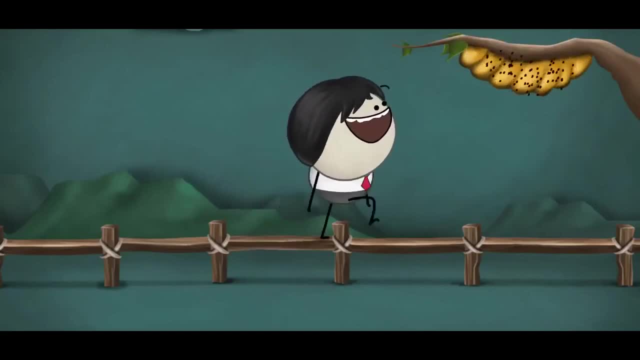 Okay. Hold on. Don't go near that honeycomb. Please listen to me. It is quite dangerous. Fine. 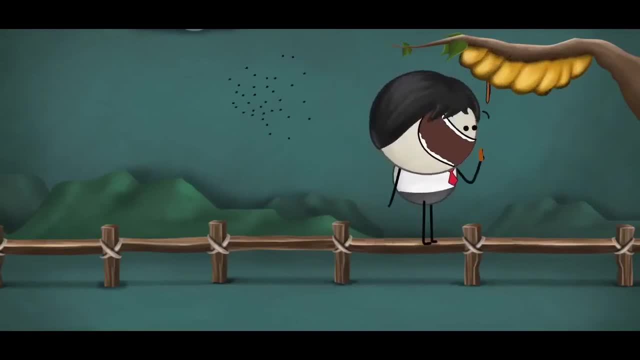 Go ahead. See I told you. Okay. Now don't worry. 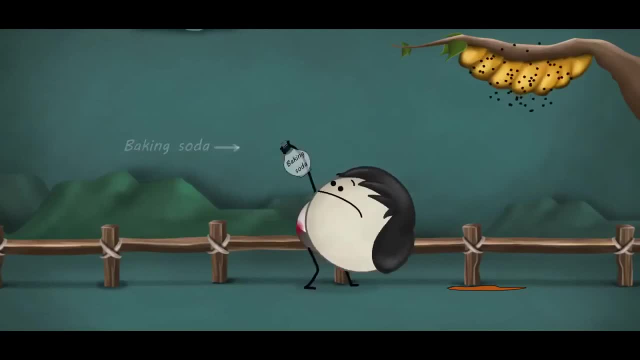 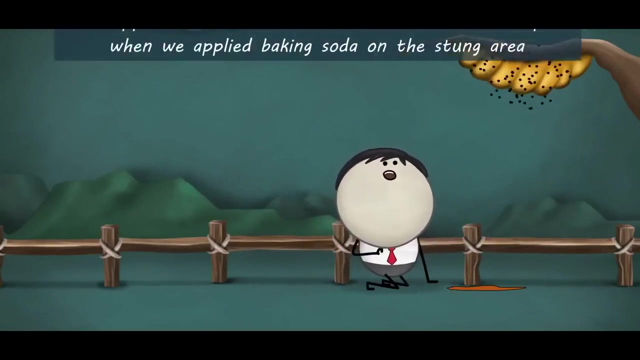 Put this baking soda solution on the bee stung area. You got some relief. Right? Do you know why you got relief? This happened because a neutralization reaction took place when we applied baking soda on the stung area. 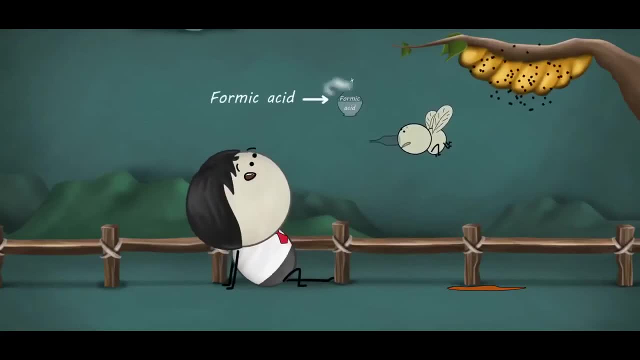 The venom of a honey bee contains formic acid. When it stings us. It injects that acid into our skin. Oh. I see. 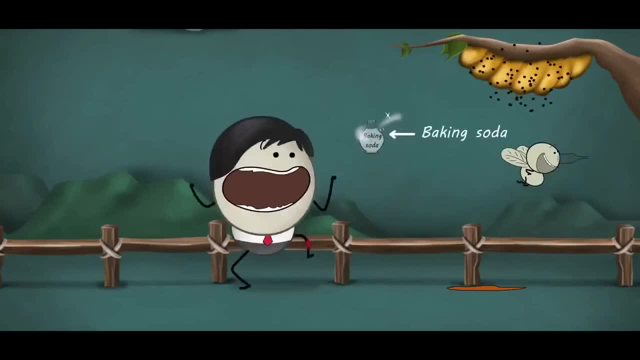 It causes pain to our skin. Formic acid causes immense pain and irritation. 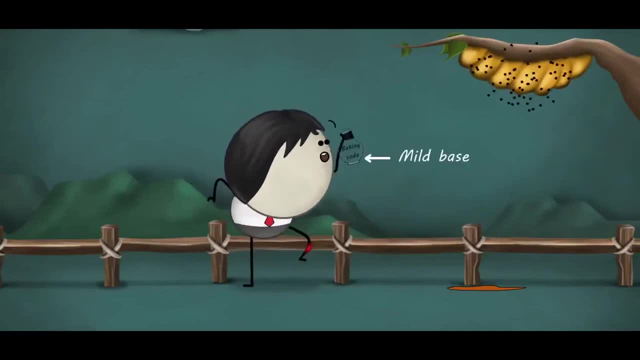 However, when we apply baking soda solution which is a mild base on the stung area, it neutralizes the formic acid and cancels its effect. 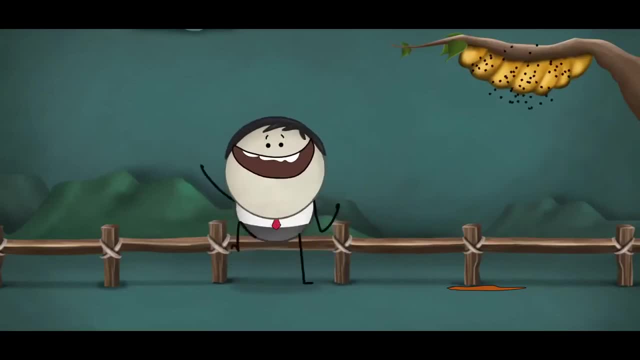 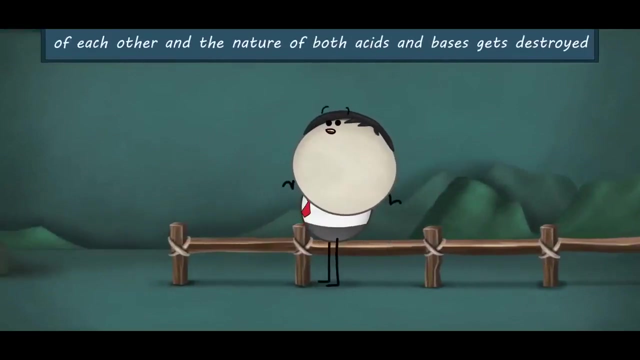 As a result, the sensation of pain and irritation decreases and we get some relief. Such a reaction between an acid and a base is called neutralization. It's over. In neutralization, both acidic and basic solutions neutralize the effect of each other. The nature of both acids and bases gets destroyed. 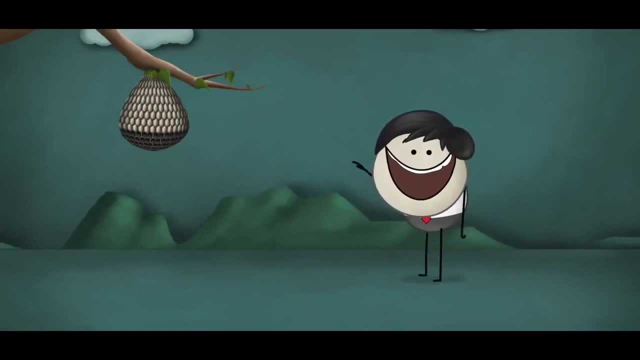 Hey, wait. What are you doing? Don't tease that insect. It is not a honey bee. 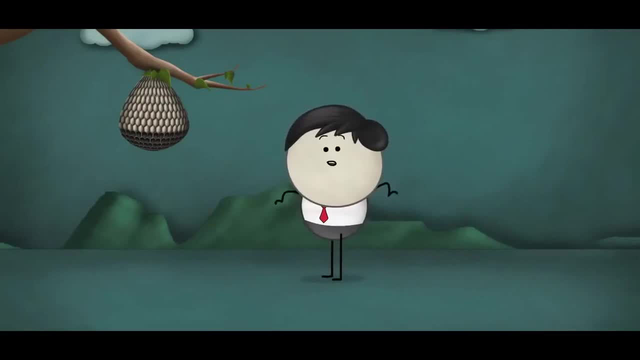 It looks similar to a honey bee but it is a bit longer. It is called a wasp. 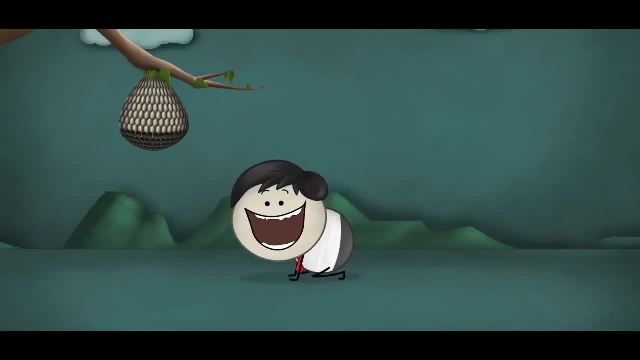 At least this time listen to me. Ok. Don't listen and bear the consequences. 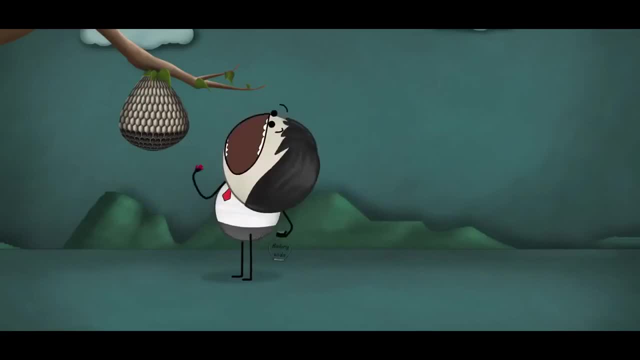 Applying the baking soda is not going to help. See. Nothing is happening. I will tell you what to do. 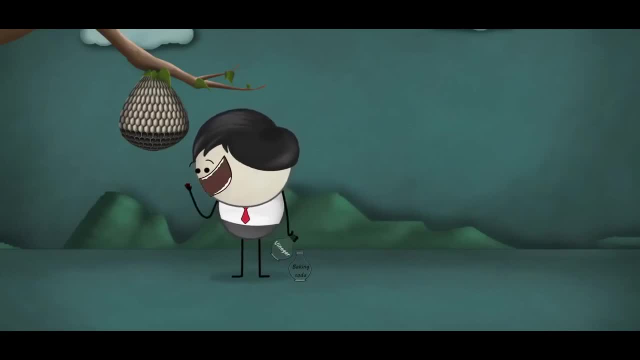 Pour this vinegar on the stung area. You will get some relief.